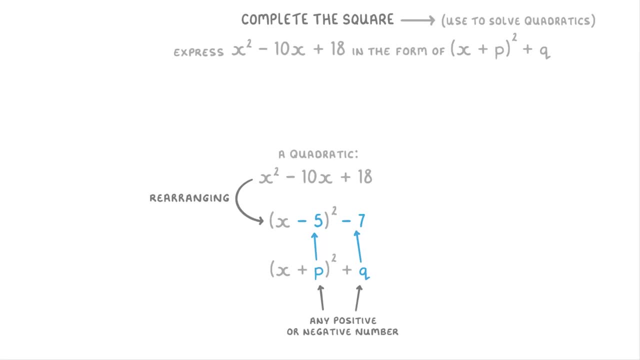 form as follows, of x plus p, squared plus q, And the fact that they're asking for it in this form is their way of telling you that you should use the complete, the square method Before we see how it works, though, I just want to say that this method is a bit weird and takes a bit of getting used to. 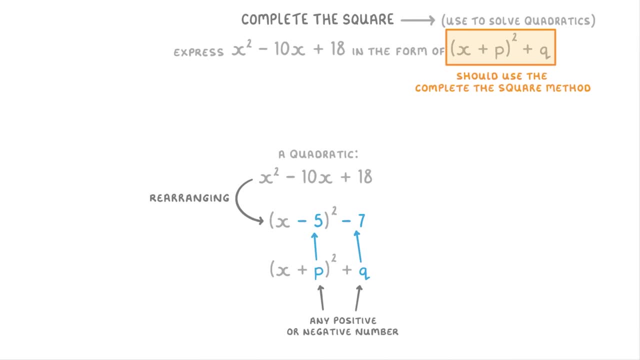 So try and follow along with the steps that we're doing in the video and then just do a whole bunch of examples to get used to it And, of course, feel free to re-watch the video as many times as you need to. So if we try it for this example here, the first thing we want to do is make sure that. 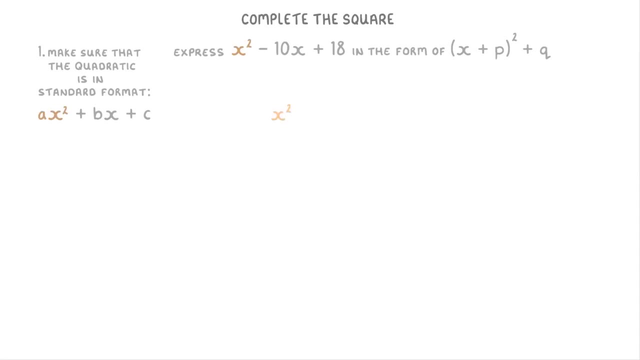 the quadratic is in the standard format, with the x squared term, then the x term and then the number term, which ours already is. So a is 1,, b is negative 10, and c is 18.. Next we need to plug our values into this formula here. But the weird thing. 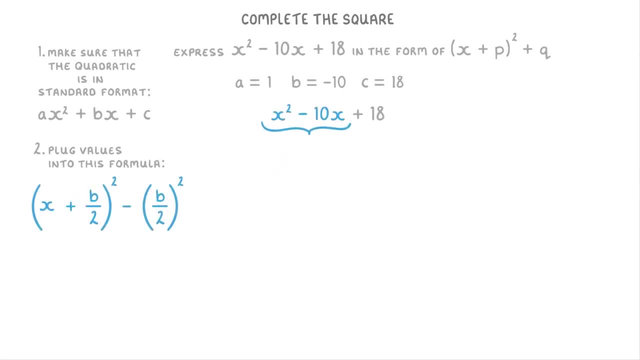 is that this formula only helps us to rearrange this first part of the equation with the x squared and the x terms. We leave the c value, which remember is 18, alone for now and we come back to that later. So in this question, because b is negative, 10, 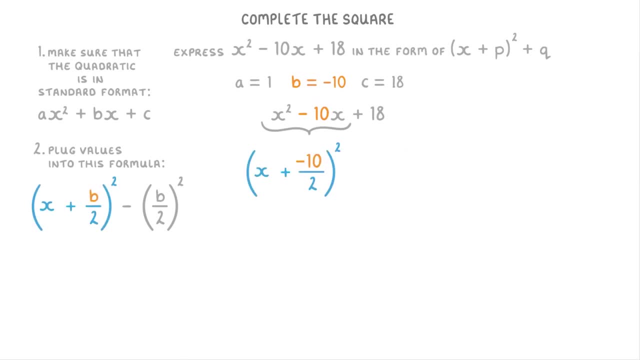 we're to do x plus negative 10 over 2, all squared, minus negative 10 over 2 squared. Remember, though, this formula is only equal to this x squared minus 10x section above. So to make the equation complete, we also need to take our c term, the 18, and add it on to the end. 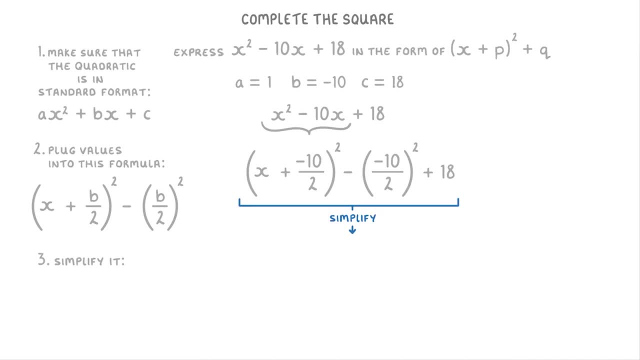 Then the last thing we need to do is simplify it all as much as we can. So because negative 10 over 2 is negative 5, we can simplify it to x plus negative 5 squared, which is just x minus 5 squared, and then minus negative 5 squared, which is minus 25.